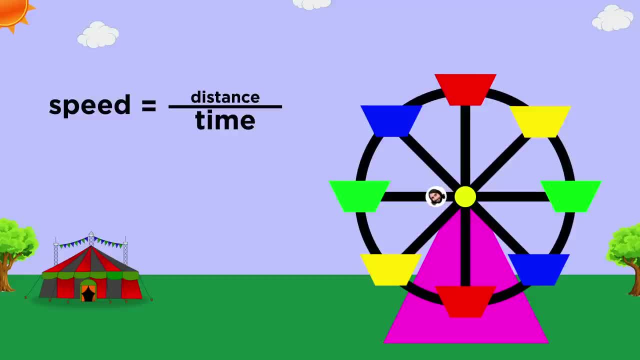 Since speed is distance over time, a shorter distance covered in the same amount of time must mean a slower tangential speed. This seems counterintuitive, since the wheel is one object, but that's why we can also discuss angular velocity, which we will learn about later. 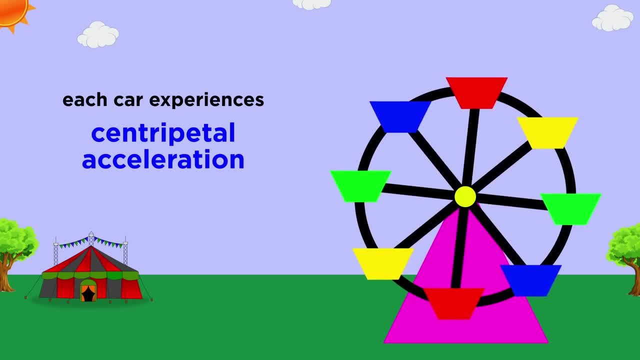 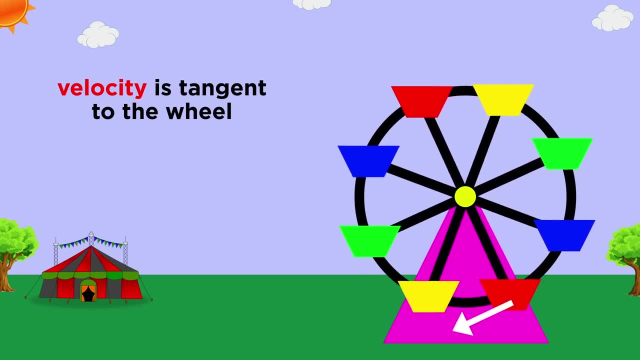 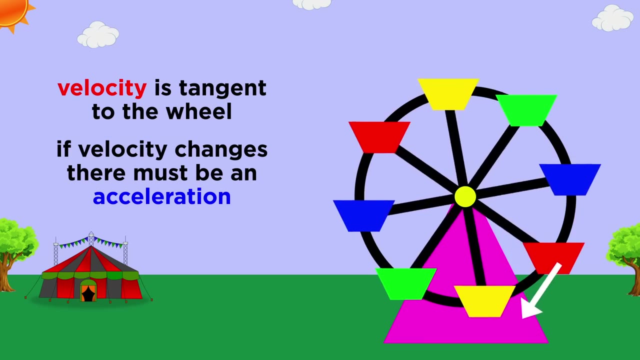 Uniform circular motion of the car happens because of a constant centripetal acceleration towards the center of the wheel. At any given moment, the car has a velocity vector that is tangent to the wheel and, while the magnitude of this velocity will not change, the direction is constantly changing and 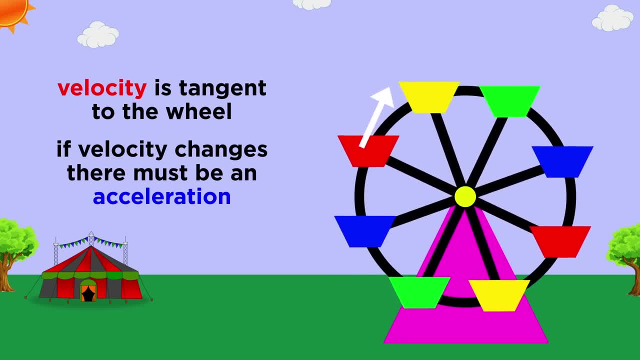 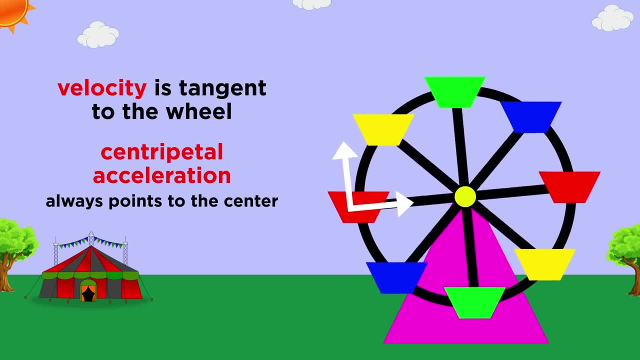 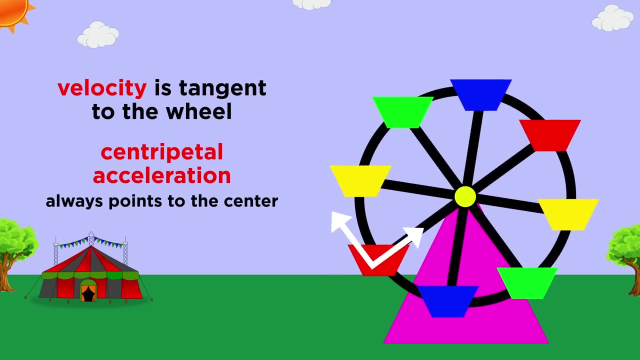 any such change in velocity can only happen due to some acceleration. The centripetal acceleration will always point towards the center of the wheel, which will, in turn, continually change the direction of the car. This is called tangential speed. This is what produces the circular motion, as though the car is always trying to move. 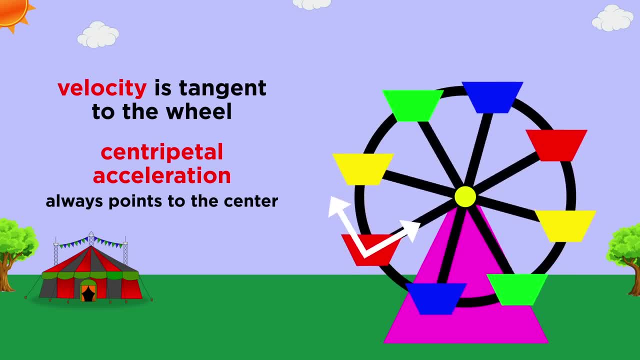 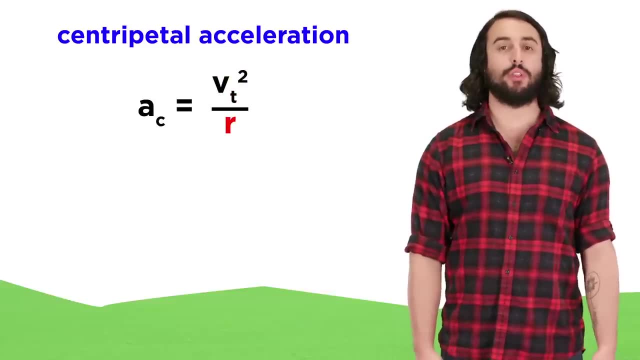 towards the center of the circle, but never makes it there because of its tangential speed. Centripetal acceleration is given by tangential speed squared over the radius of the path, so this value would increase if the car were to move faster and if it were to sit closer. 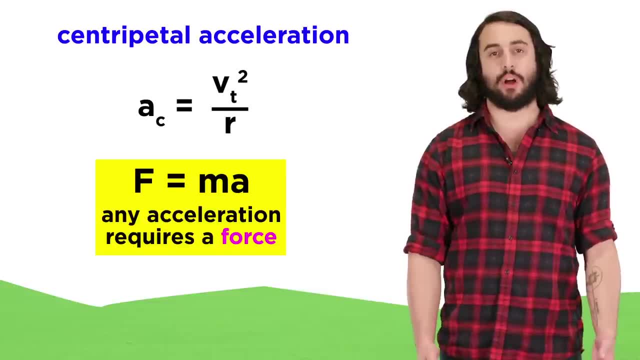 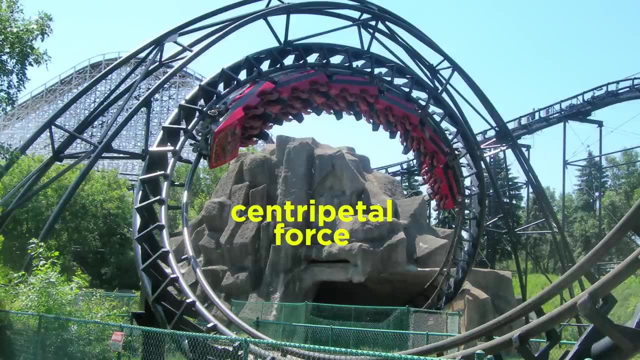 to the center. We know from Newton's equation that the velocity of the wheel is always constant. We know from Newton's second law that if an acceleration occurs, there must be some force present to produce it, and centripetal acceleration is generated by the centripetal 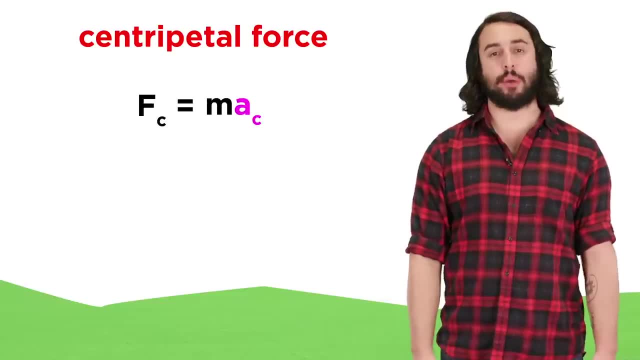 force. Centripetal force is simply centripetal acceleration times the mass of the object, since F equals m, a. So we can describe centripetal force by simply adding the subscript c on force and acceleration, or it can be given by m times tangential speed squared over the radius of the path. 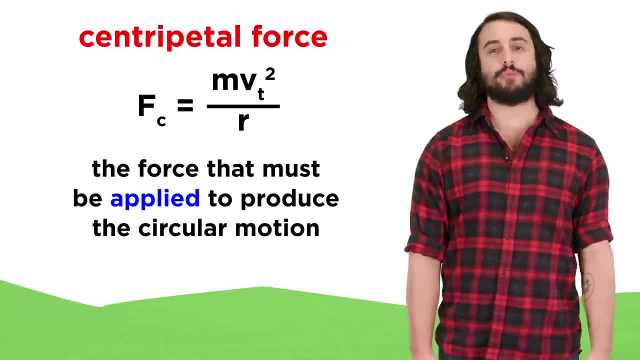 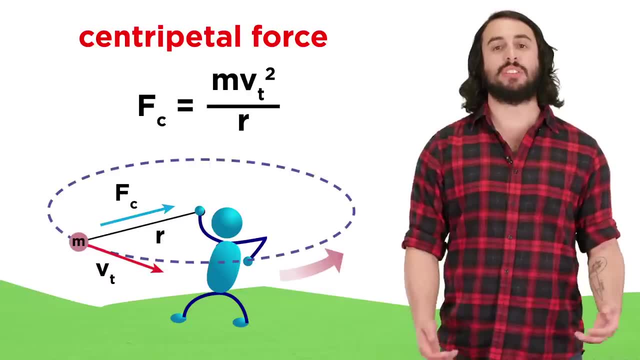 At any given moment, the car is always continuing to turn and if the car is always contracted, it will always continue to turn of the path. This represents the force that must be applied to produce the circular motion, like the amount of force that must be applied to spin a ball on a. 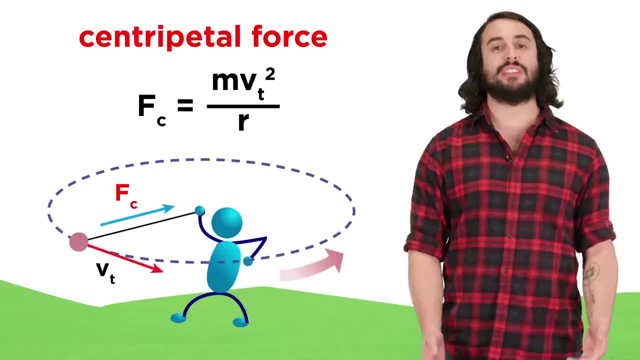 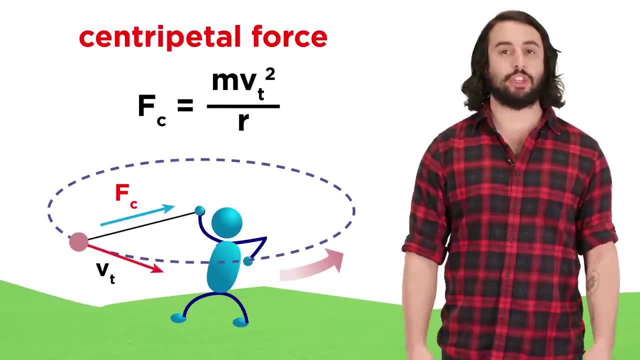 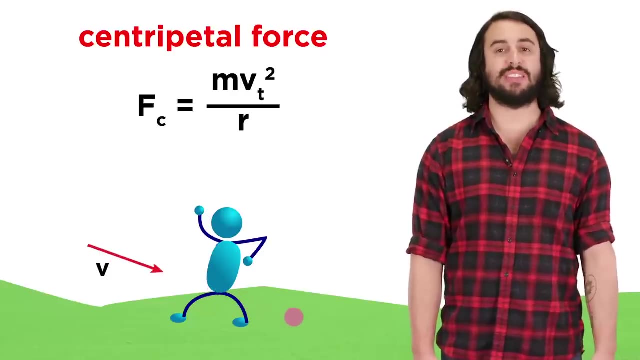 string in a circle around your head. If this centripetal force that points towards the center perpendicular to the tangential velocity, were to suddenly vanish, in the event that you were to let go of the string, then the object would simply move along the tangent line at the precise moment of release, since